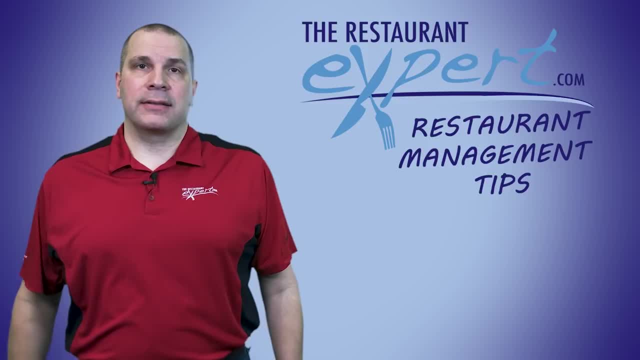 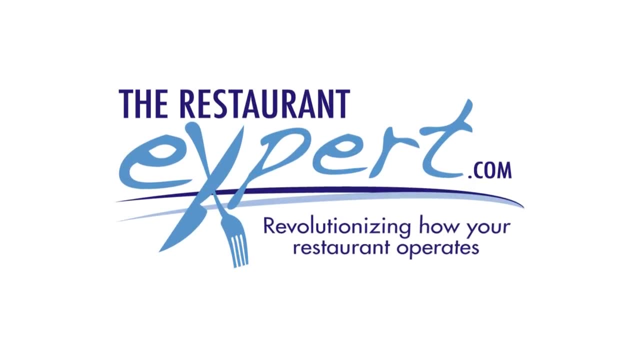 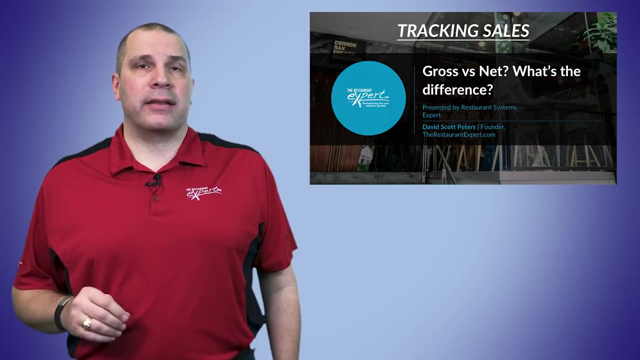 one and why you should use one over the other in just two seconds. Hello, this is Dave Scott Peters with restaurantexpertcom And, heck, I got to tell you this. It's confusing out there, You could read blogs, articles, listen to webinars and so on. 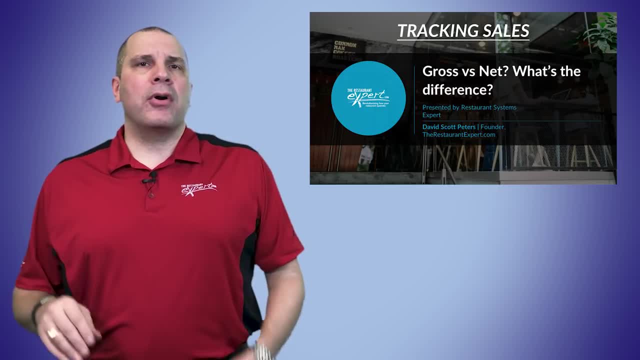 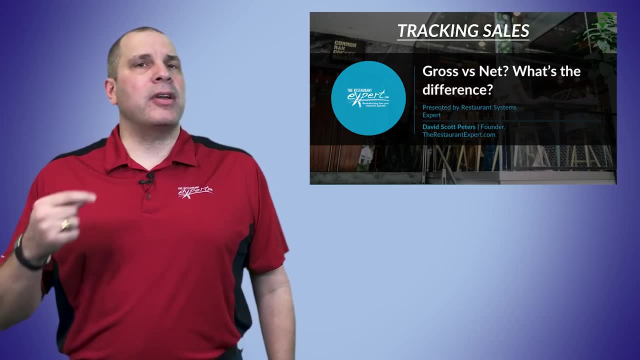 and you're going to find industry experts that use one number over the other when it comes to gross versus net sales, when calculating cost of goods sold and labor cost. Now I'm going to tell you what goes into each and I'm going to tell you what I recommend and why. Number one there's 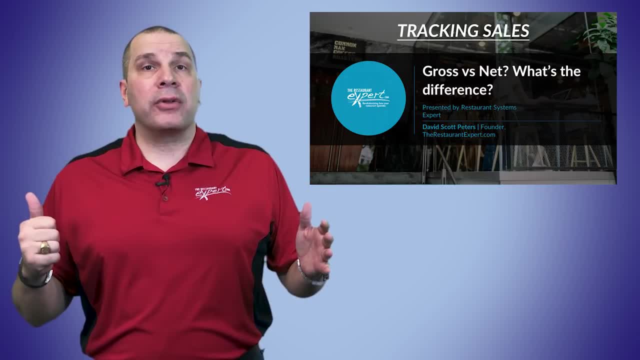 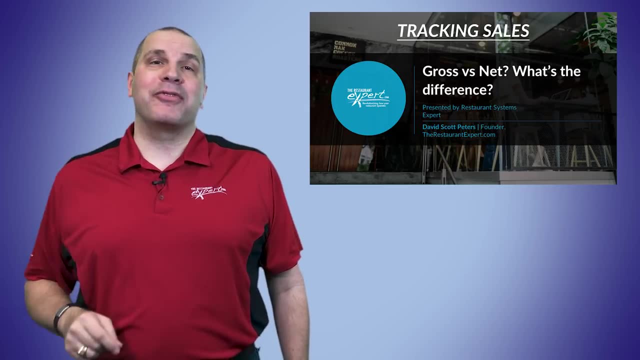 gross sales: the ring of the register before discounts, not including sales tax. Sales tax is not a sale. It's the pleasure the government gives us of holding their money and penalizing us like the mob. Don't give it back to them, Don't use their money. So, gross sales. ring of the register before. 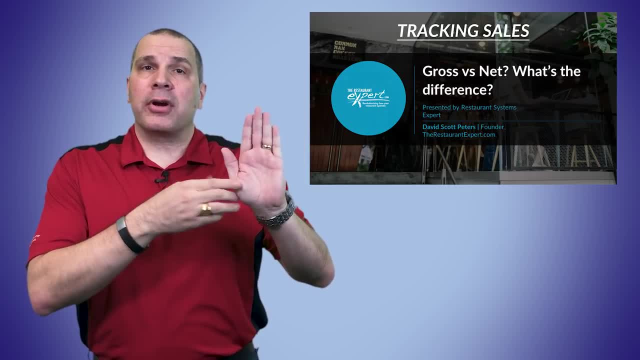 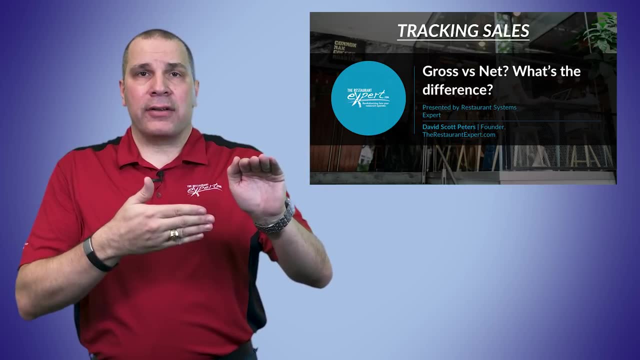 discounts not including sales tax. So if I ring up a $10 burger comp $5, gross sales is $10.. Net sales is the ring of the register after discounts. $10 burger minus $5 discount: $5 is net sales. 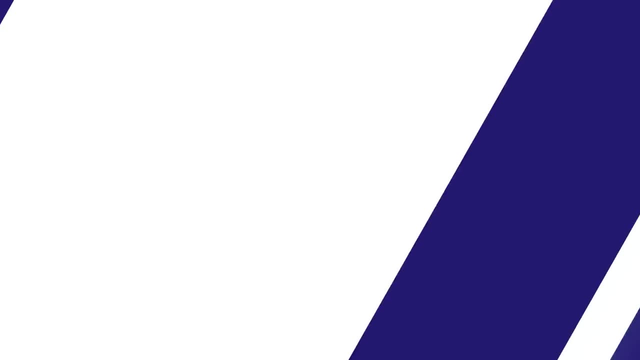 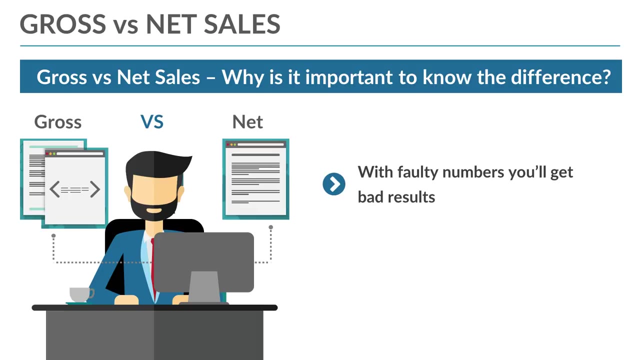 Again, sales tax is not included. It's not a sale. So what do I use? $10 burger, $5 comp. use gross sales to measure my cost of goods sold or, as many experts say, net sales after the discount, because that's truly your food cost. Well, 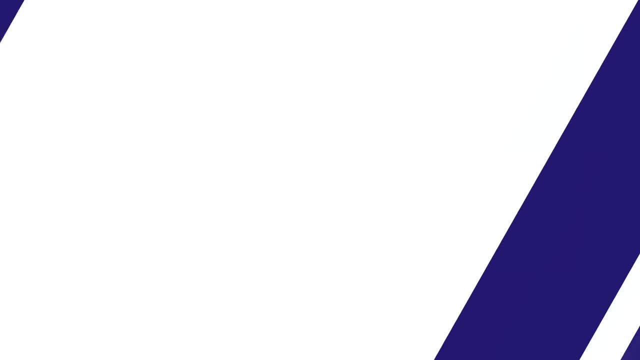 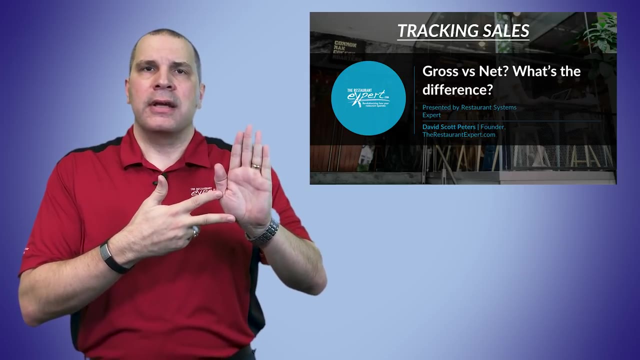 I'm going to tell you right now it's gross sales, Because here's the deal: I asked my chef to put a burger out for $10, use $3 in product use, divided by sales, 30% food cost If I discount $5 on that. 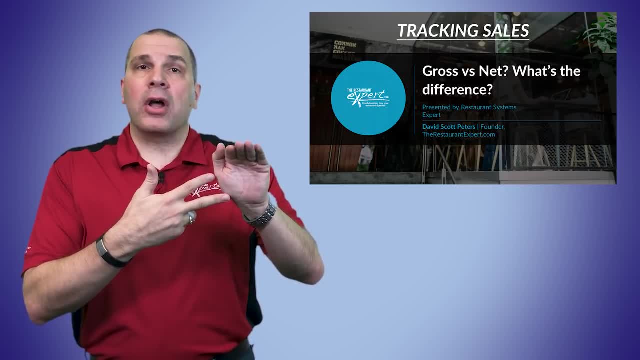 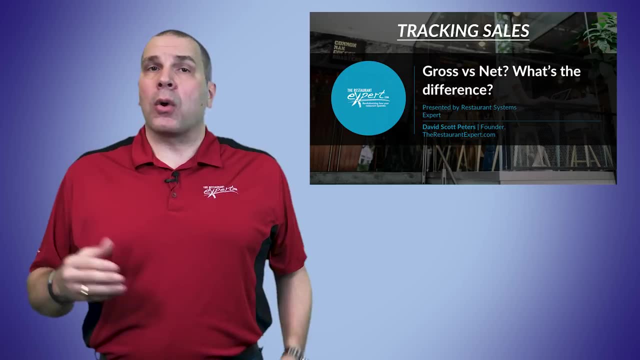 burger. what happens to my food costs using net sales? It's no longer 30%, it's 60%. It's that chef's fault that you decided to give away. run a BOGO, buy one, get one free Or, worse yet, run a. 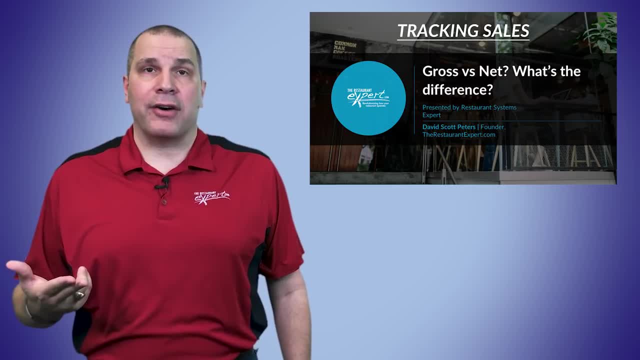 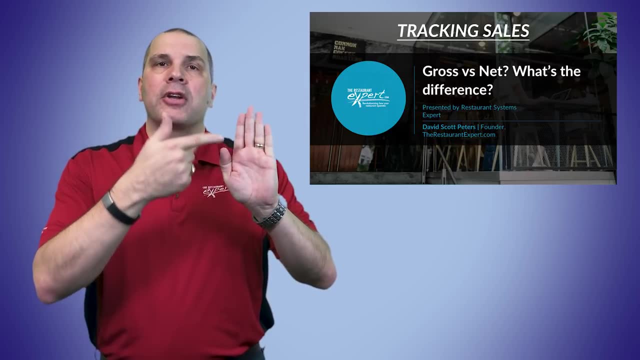 Groupon at a 78% discount. Just kill yourself, right. So I'm going to measure my chef. I said: chef, sell it for $10, use $3 in product. That's a fair measurement. gross sales Still not with me.